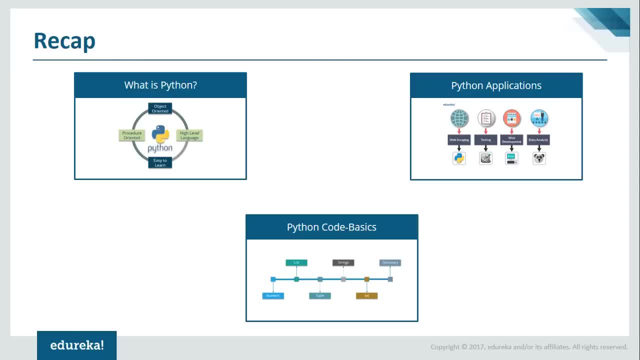 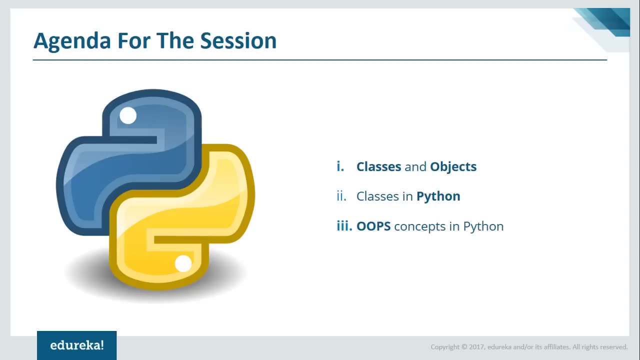 we looked at the various applications which were built using Python in different domains as well, and then we moved on to the Python code basics, wherein we spoke about the different data types, the different data operators. we saw conditional statements, we saw a little loops and so forth. Now in this session, what we'll majorly be talking about are 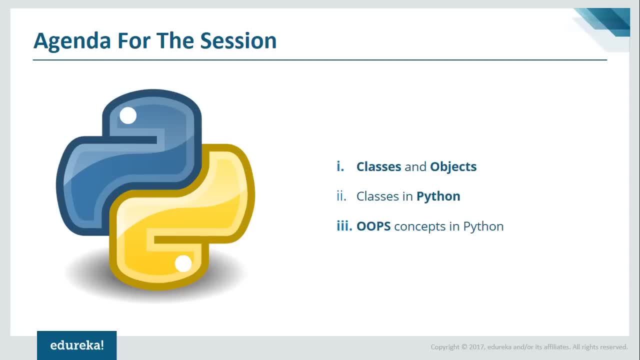 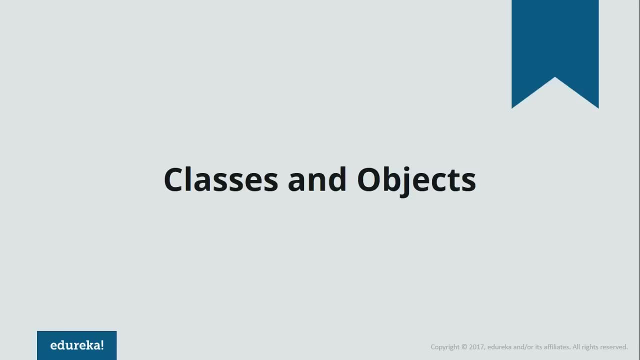 classes and objects: classes in Python and object oriented concepts in Python as well. Now let's first start about classes and objects. Now, to those of you who are not familiar with the different programming paradigm, two of the most programming paradigm is object. 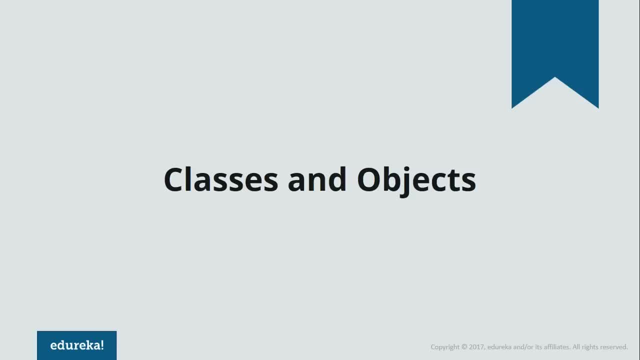 oriented programming and procedure oriented programming. Now, when you look at older programming languages like C or C++, you'll notice that there are a lot of different programming languages. Now you can see Visual Basic as well. These follow procedural oriented programming language style, wherein what used to happen was that the entire program was 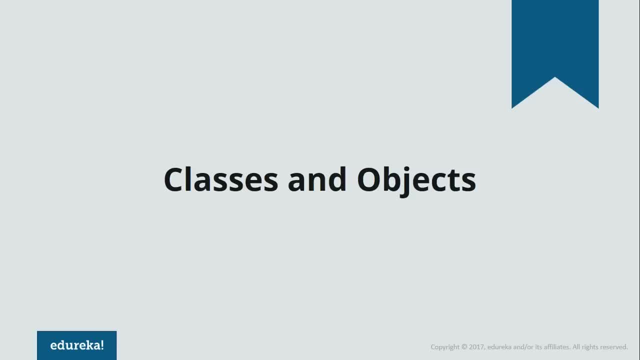 divided into smaller parts, known as functions, and the importance was not given to the data, but the sequence of actions which were performed. Also, what used to happen there was that the entire process took a top-down approach as such, But what happened is when newer programming 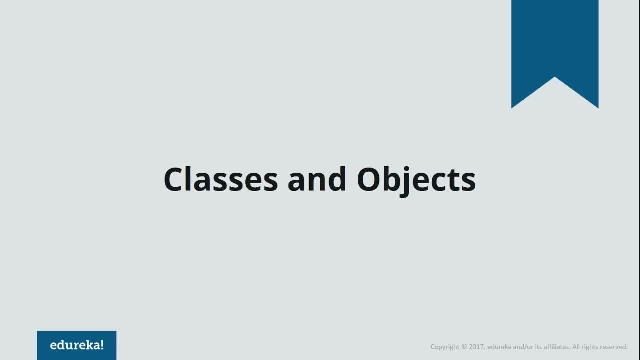 languages came up, they realized the value of the data and they were able to use it in order to create something known as objects. Now, objects are quite similar to what you can relate to in real-world entity as well. Now, anything that we see around, anything that has different, 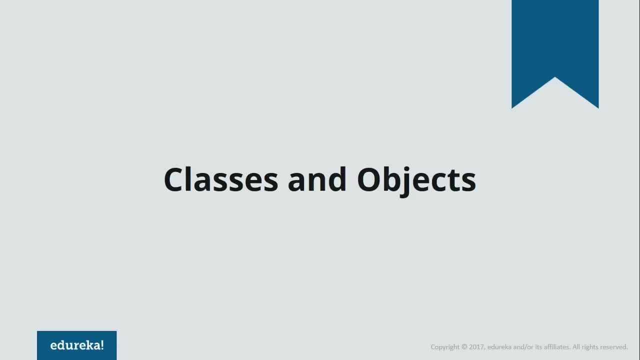 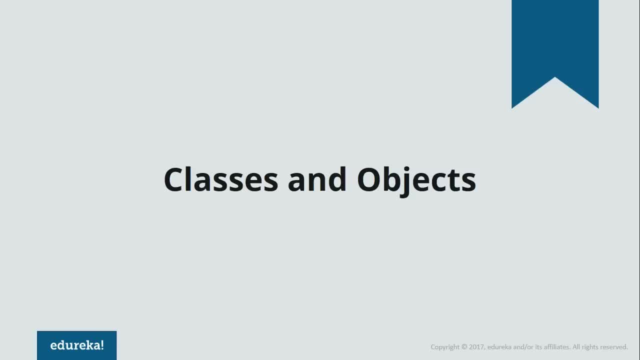 security, as well as more and more elements, mana, and you can use various operations like data accessing, data overloading, data expansion and so forth. Now, some of the examples of objects oriented programming languages is C-Sharp, Java, visual basic, dot net and so. 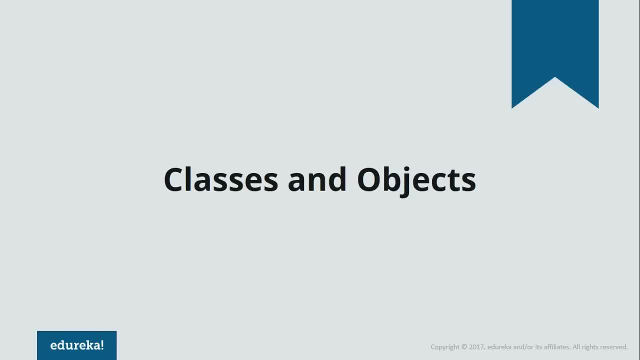 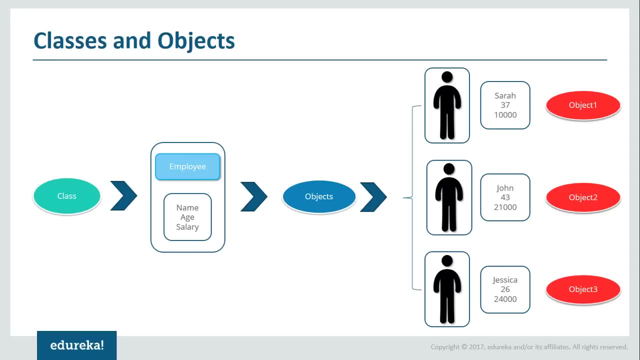 forth Now. let's first address the question of what exactly is a class, an object? Now, to help you understand this better, Let's actually look at an example here Now to give you a simple, one-line definition. a class, basically, is logical grouping, which would 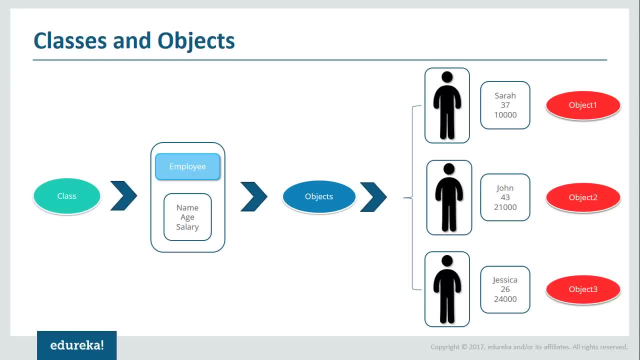 helps us reuse and rebuild our data as part of the code. Now, to put it quite simply, it basically is similar to a template or a blueprint that we use. Once I have defined a specific requirement of mine, then what I can do is that I can go on variating with respect to that. Now let's look at 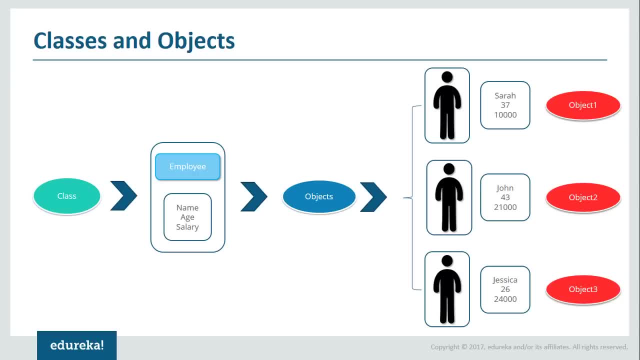 the example here. Now, if you look here, I have created a class called employees, wherein I have defined some of the most common parameter each of my employees will be having: There would be his name, there would be their age and there would be their salary. Now I have defined a blueprint, but 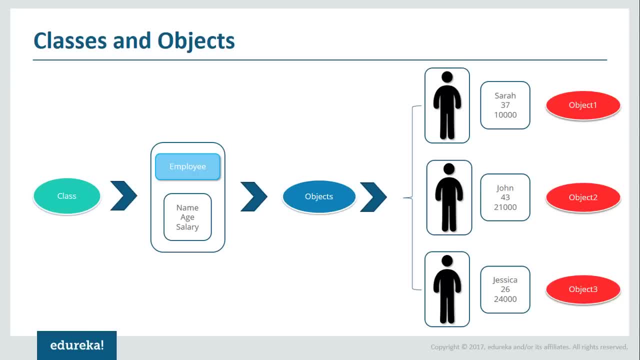 there comes a time where I need to implement this, So an instance which is basically an entity of the class is referred to as an object here. Now, if you look here, there are basically three different objects. I have object 1, which is referring to Sarah, whose age is 37, as well as salary is 10,000. 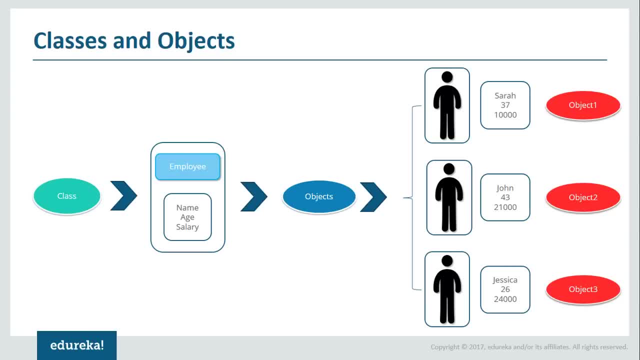 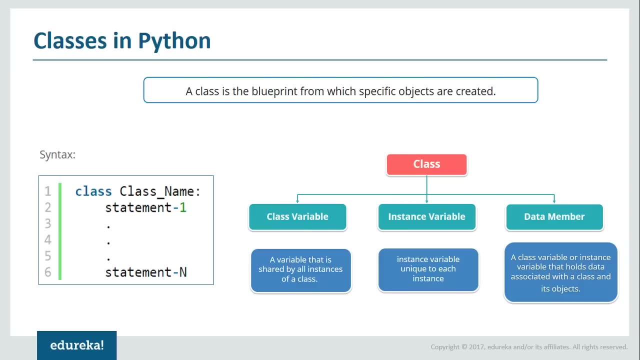 My object 2 is John, whose age is 43 and salary is 21,000.. Similarly is Jessica as well, whose age is 26 and the salary is 24,000.. Now, how does Python implement classes? Now again go back to the definition. A class, basically, is a. 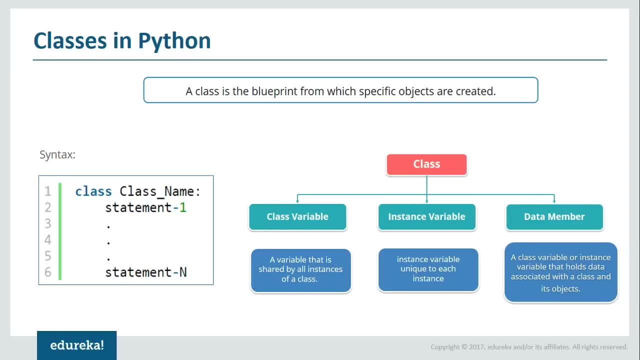 blueprint for which objects are created. Now, coming to the basic syntax for how to write a class in Python. it's quite easy, because you just need to define the keyword class, following which you need to specify the name of the class. Now let's go. if you take the previous example, the name of that. 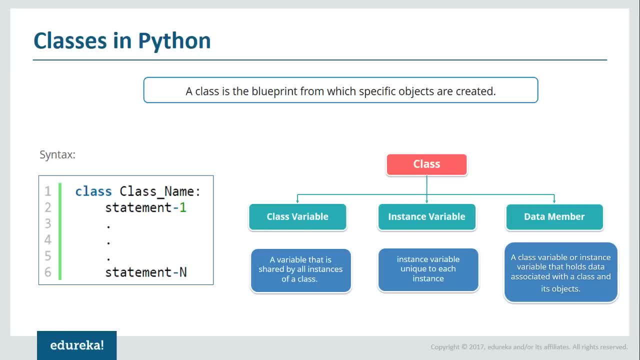 class would be employees and each of the objects would be created from that same class. Now, what I'm going to be writing inside the class would be three major aspects: I would have my class variables, I would have instance variables and I would have data members. Okay, now, these are the three major 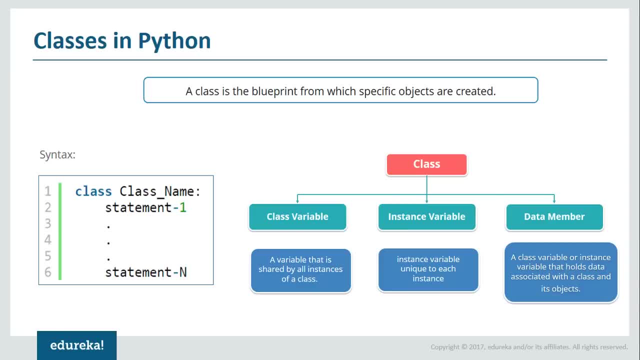 aspects to any class as such. Now, if I need a variable which is going to be shared by all the objects. Now do not get confused: when I say instance, It basically is referring to a object itself. So here we refer to an object as instance, Now each, if I want each of the instance to share a. 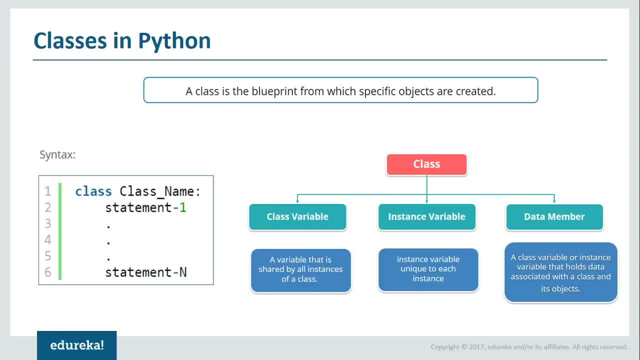 common variable, then I would make it a class variable. But let's say I want each of the instances to have a specific variable. Okay, then I would be using an instance variable as such. Then comes the third part, which basically is your data member. 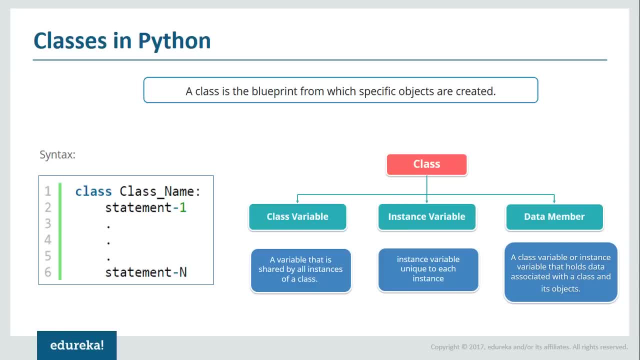 This is a class variable, or an instance variable as such, that actually holds the data associated with respect to the class and objects. Now, without confusing you any further, let me actually switch to my PyCharm. Okay, and let me show you this by writing, by defining a class here itself. Okay, so, 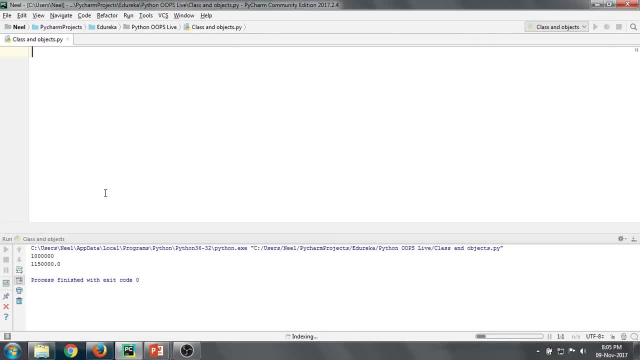 if you guys can see my PyCharm. can you give me a quick confirmation in the chat box? 기�jug, Okay, I seem to get a lot of confirmations. Thank you, guys. So let's start by creating a simple class Here. now let me use the first key word for defining any class, that is, class. 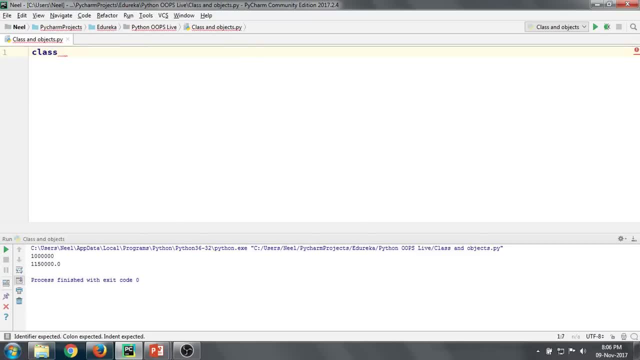 then comes the name of the class. Now for today's example, what I'll do is I'll create a class called cars. Okay, So I've created a class called cars, okay, can you guys see this? okay, and here, what I'm going to do is that right now, I'm not going to write. 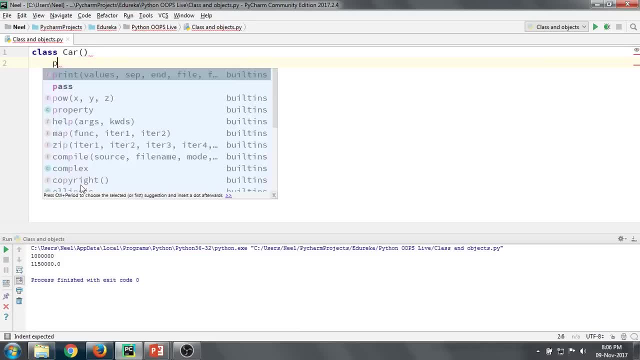 anything. so I'm just going to use the keyword pass. then comes the time for me to create objects for this class. so what I do is: let me call an object, let's take an offer out, okay. so this is the name of my object, and then I'm going to specify. 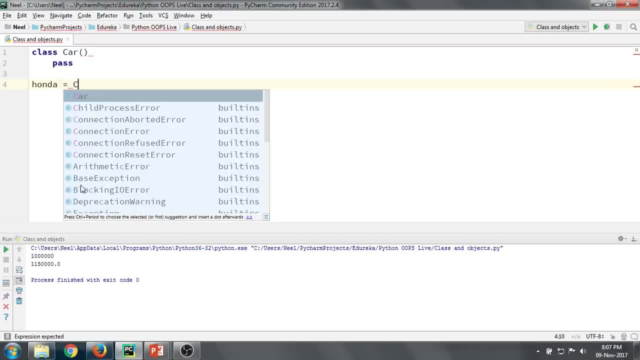 to which class it belongs to. so it belongs to the class car, and this is how you create an object in Python. quite easy, right. similarly, let me create another one. let me call it start: okay, Tata is also going to be of car, okay. so basically, what I have done here is that I have created two objects that 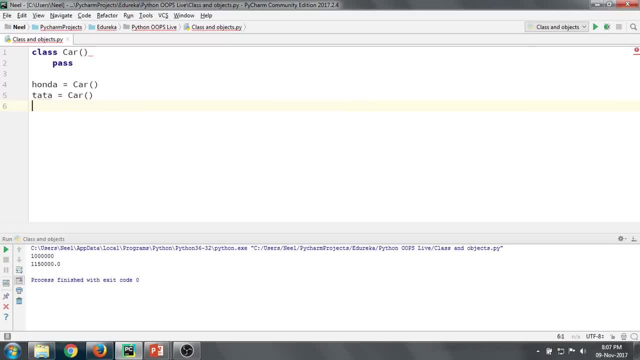 belong to a specific class. now time, now comes the time when you actually are assigned values to these instances or objects as such. now let's see, I want to add the name or the model number for the Honda car, so I'm going to say Honda, which is my object, following which use a dot operator and then specify what. 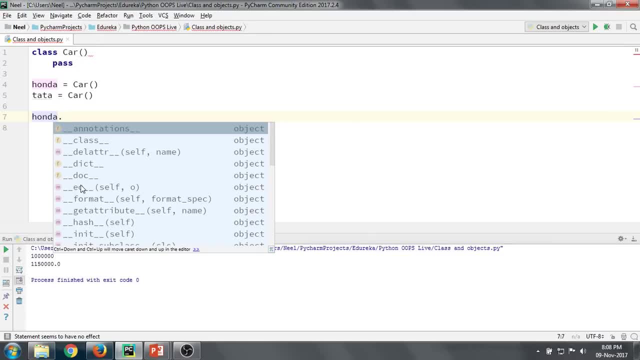 instance variable you want to use. now, let's say I want to specify model name. okay, model name is equal to, I'd say, city, because I like Honda City. okay, now I'll also add another variable, which is year of manufacture. so I'll say year M, okay, and this, basically, is going to be. 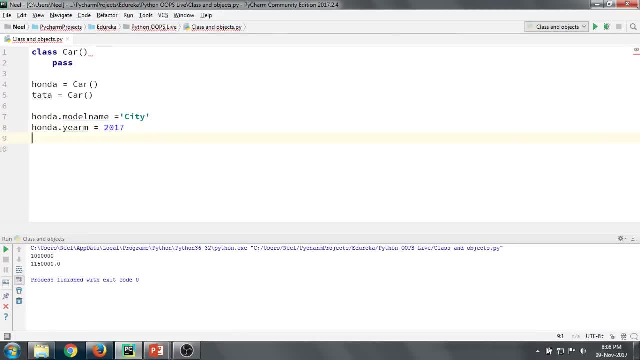 equal to, let's say, 2017. now I'll also add price. okay, I'd say about 10 lakhs. does that sound fine? now let me just copy the same and let me create an object for Tata car as well. now, here, let me just change it to Tata. 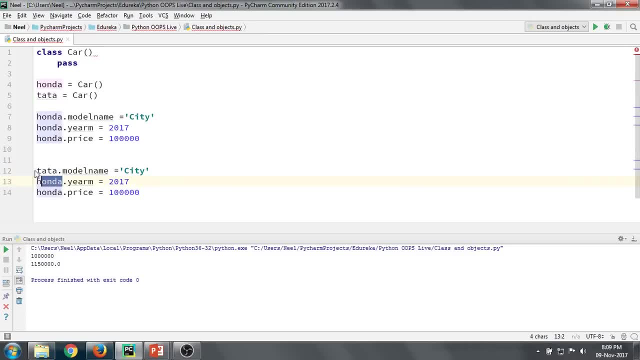 and let's say: this is bold. okay, so let's keep the year the same, or let me reduce it to 2016. and let's say: the price is: let me reduce it, I'll make it six. okay, does that sound fine? now, what I have done here is that I have created. 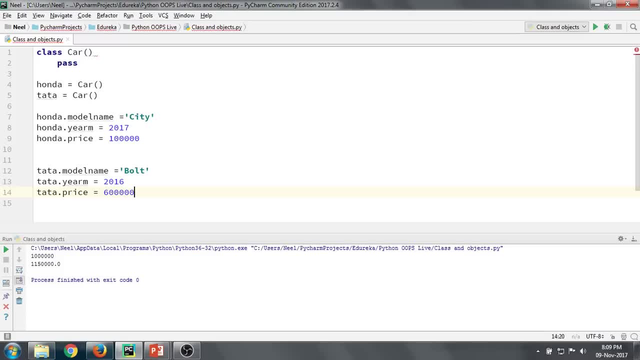 instances of the class or objects to that class, and each of these instances themselves have a specific variable assigned to them as well. so in this case, what you see here is the model name, what you see is the year and what you see is the price. so these are basically variables associated to each of these. 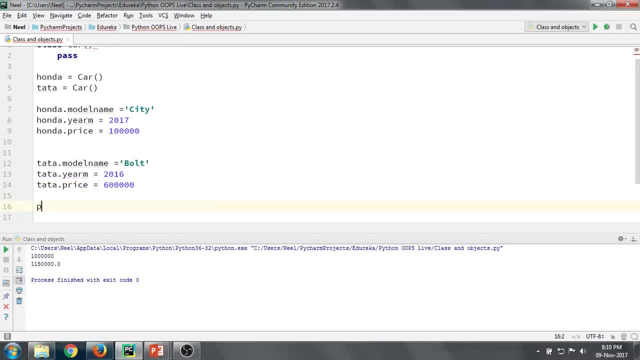 instances as well. now, if I say just print and I say Honda dot model name, okay, let me take the price itself. let's try running this. ah, you see the mistake here. can anyone guess what's the mistake here with respect to the price of the car? let's try running this. you see the mistake here. can anyone guess what's the mistake here with? 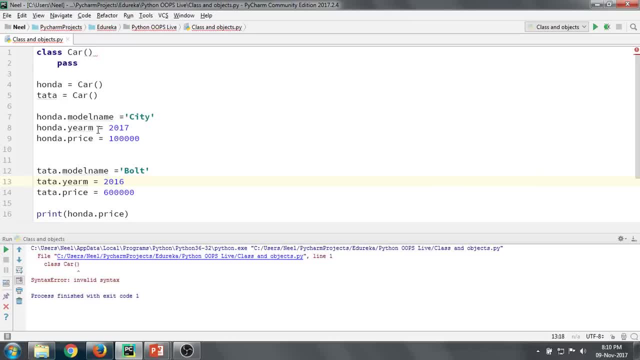 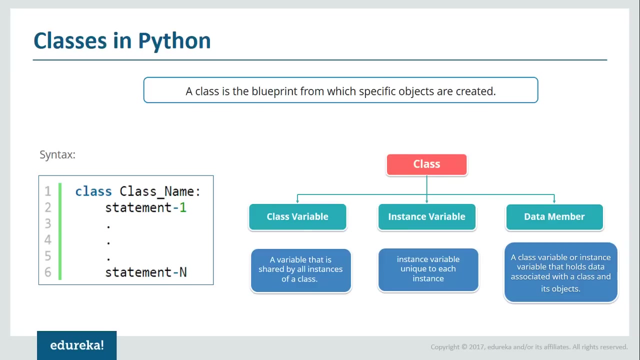 respect to the code. okay, it's with respect to the definition of the class. now, if you go back to, if we go back to our slides here, can you see there's a small semicolon here that we have missed out. so this is how it is. a single semicolon can make a lot of. 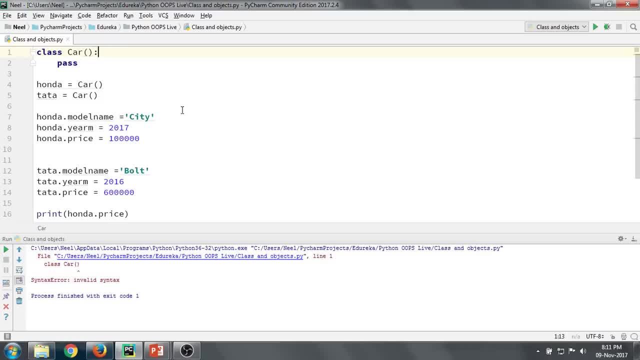 difference. okay. okay, now let's just save this, let's run it. ah, okay, I can see the price of my Honda car here now. this is a lot of pain for me when I'm working with multiple instances which have unique variables to them, but let's say, if I have common 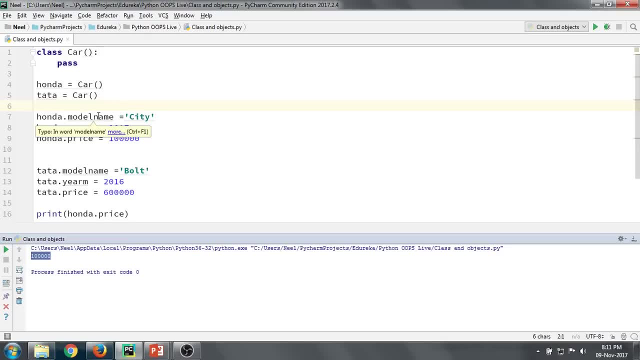 values that needs to be created for all of these. if I was using other programming languages, we had a concept known as constructors, but don't worry that same is present here as well, with Python. So to create a constructor, use the following command, which is def, which is basically defining a function, and use init. Now, init is basically a constructor here. 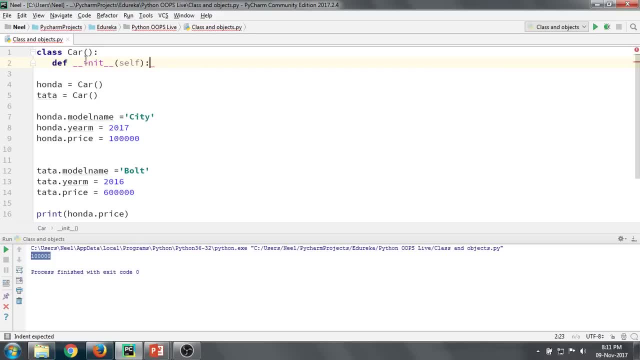 and what it is representing is that it is going to initialize the value of the variables. Now, if you notice, here there's a keyword that is already added here, that is self. Self, basically, is a reference to the object which is going to be calling this function. Now, those of you who are 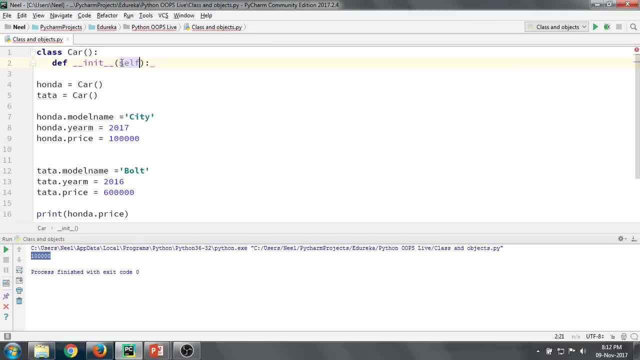 not familiar with functions can check out our video on Python tutorials, where we have talked about functions, and also check out our Python function video as well. Okay, now what happens is to this: let me pass a model name. I'll also pass the year, manufacture and let's say the price as well. Okay, now I need to. 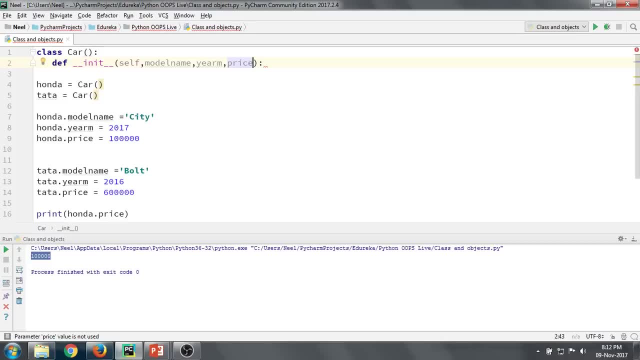 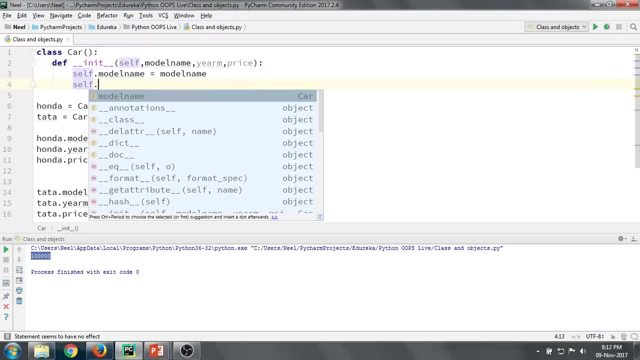 assign the values for these variables for all the object. Now, if I need to do that, then what I need to do is that I need to first reference the object, So that's selfmodelName, equal to the model name that it's getting, So then selfyearOfManufacturing. 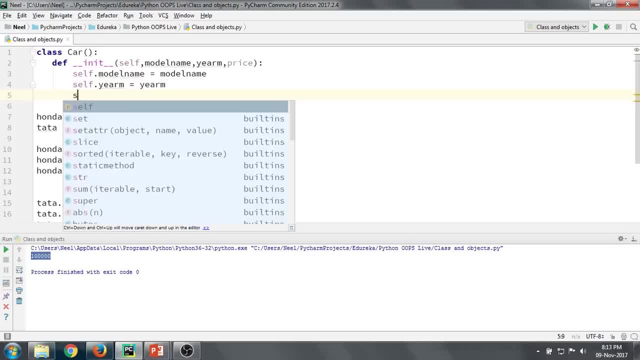 and finally, selfprice. Okay, now, what I'm basically doing is that for my constructor, I would be passing these three parameters. So, for the object or the instance which is going to be created, please add these values for that. Okay, now let me show you how to change this as well. Now, I don't 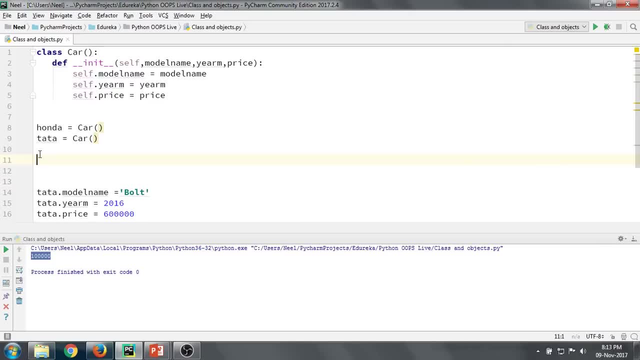 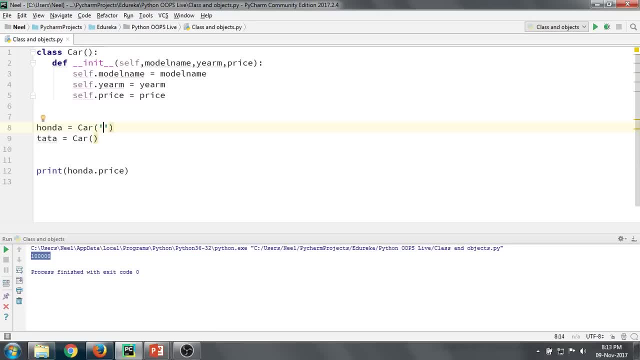 I'll pass Honda, I'll pass city. Okay, I'll also pass the year of manufacturing is 2017. and let me pass the price again. Same for Tata. So what I've basically done is that I've generalized the requirement that I want. 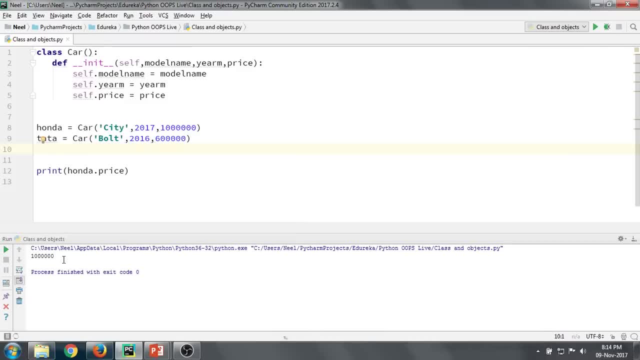 Now again, if I run the same, what you can see here is I'm getting the same output that I had gotten earlier as well. So this, basically, is a constructor that is going to be used when I have assigned specific values to my objects or instances at the time that they are creating. 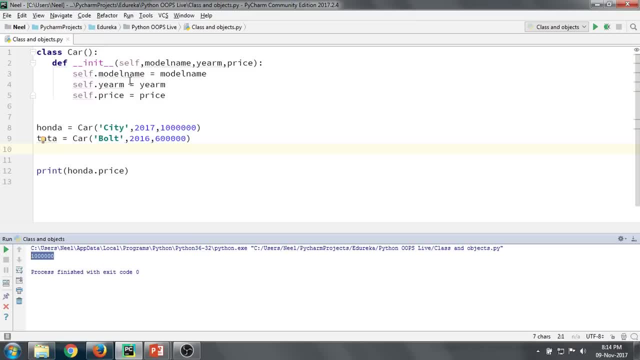 Apart from this, if you want to create or you want to add any specific value, you're free to do that. Now, let's say I want to add a new value. Let's say I want to create Honda dot. Let's say I want to add the CC as well, The CC of Honda city, which is equal to 1500.. Okay, so this is also. 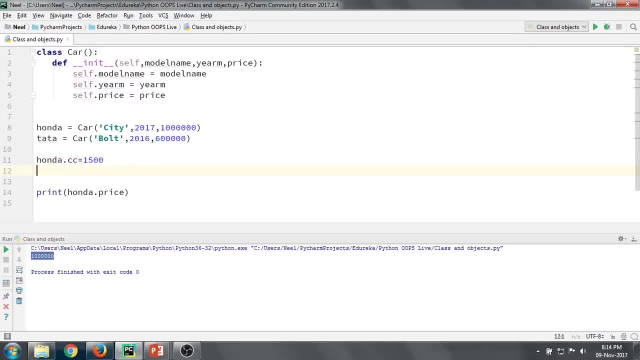 very simple. Now, what happens here is that I've created an instance variable for the Honda object. Okay, now same thing. Let me just say, if I want to see the complete values that are associated to an object, then what do I do is that I check the namespace. 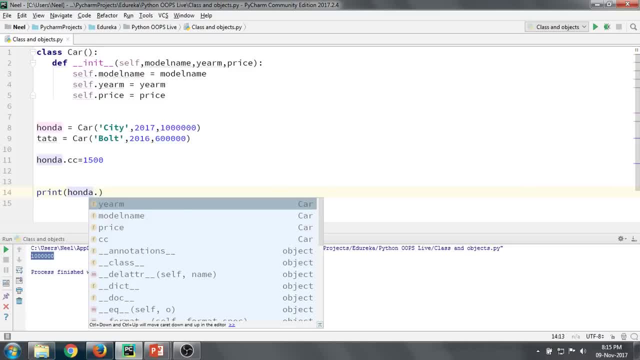 for it. Now, how do I check the namespace, for it is that I use the dictionary option. Sorry, I use a dictionary function. Okay, so if I use dict function and if I run this, Then what you see here is that I have a model name which is city. I have a year of manufacturing. 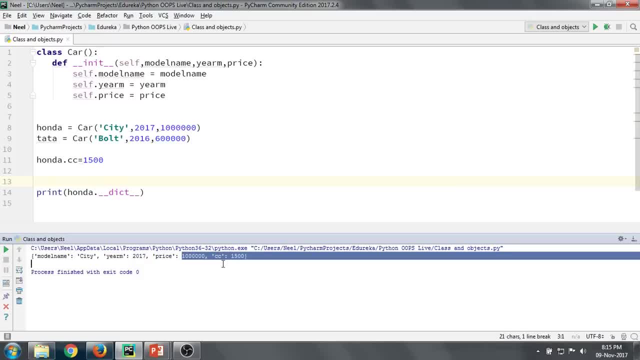 2017.. I have a price and I have the CC associated asset to it as well. Okay, now what basically it tells me is: if I use this object and request any of these values, then this is the output that I would be getting, Same if I change for Tata. 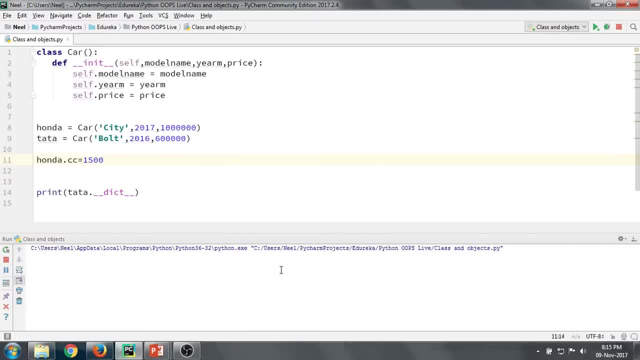 And I run this, Then what you see here is that CC is not present. So I hope you understand the difference between both. Can I have a quick confirmation in the chat box? Okay, that's great. Good to see that all of you are following it. Now, if I have a class, then if I 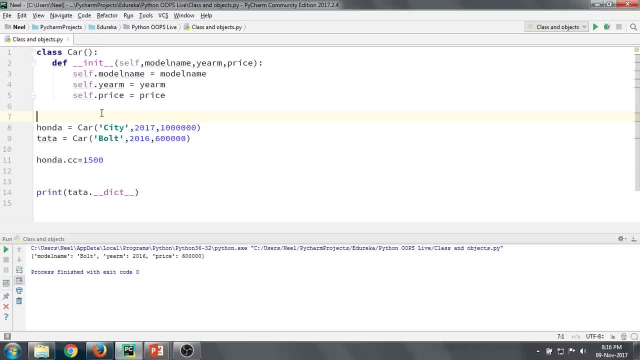 don't perform any operations in it, then I'm basically not optimizing or using the complete KPIs, So that I'm using the complete KPIs of that class as well. Now what I'll be doing is that I'll be creating a function here. So this function, what it basically does is that it's going to increase the 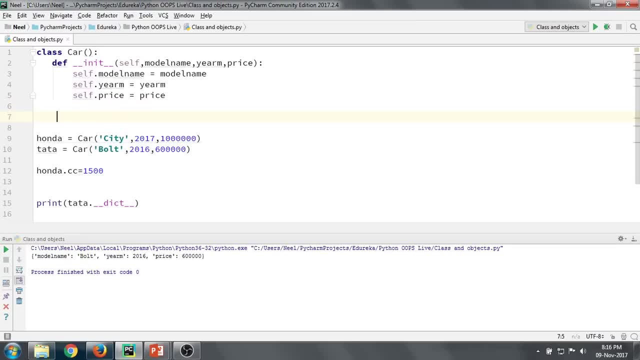 price of my car. So what I'm going to do is that, for defining any function, use the keyword def- Okay, following which the name of the function. So let's say, Price underscore increase- Okay, now, this is a function, but it's going to be performing on itself as well, so use self here, okay. 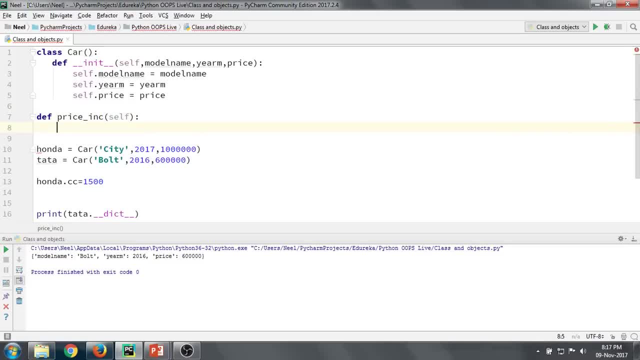 and I'm going to start defining this function. what do I need to do is that I basically just need to update the value of price. okay, so what I'm going to do is that I'm going to use self dot price equal to. then I'm going to do a simple. 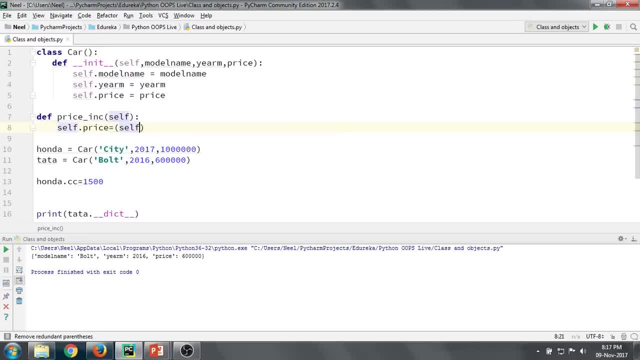 computation. let's say the present self dot price. sorry about the typo into okay, how much do you think the annual price range would be? let's take a guess. let's maybe a 15% rise. in that case, I'll go with 1.15. okay, now I have defined a. 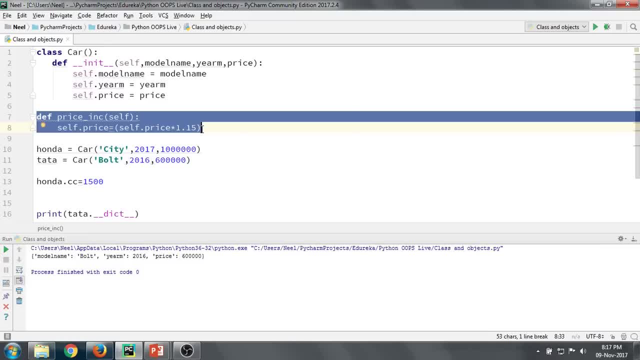 function here, but what I'm going to do is that I'm going to use self dot price. what you need to understand is that it's not exactly in the scope of the class, so, oh, sorry about that. now, how do you identify if it's in the scope or not? it's basically one of the 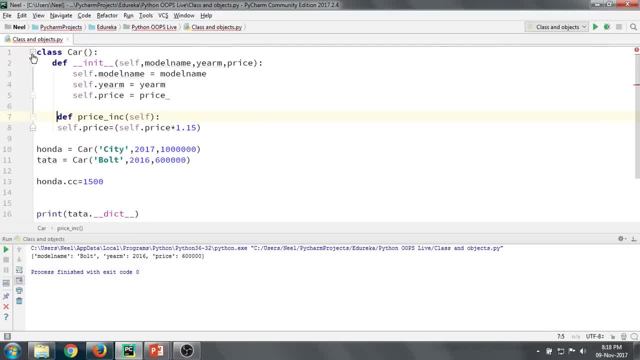 eases. with respect to pie chart, if I expand it, then I know what is part of the class and what is not. so this is one of the major reasons that we recommend you use pie charm as an IDE as such. okay, now I need to increase the price, so what I'll do is: 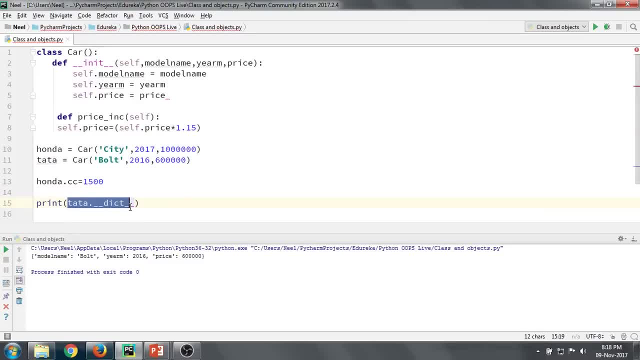 let me go back. let's say I want to check the price of the Honda first. okay, then what I'm going to do is that I'm going to call the function with respect to the class. now it's defined to that class. so what I'll do is that I'll send this. 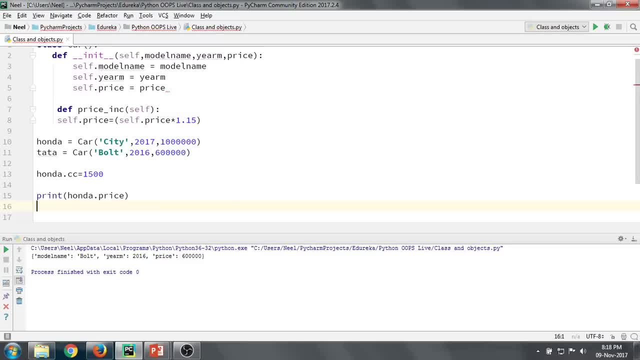 function. I'll use the Honda object to call that function. now, to use any of the functions associated to a class, make sure you're using the instance or object of that class. so Honda dot. now you can already see here the different suggestions that comes to it now. price increase is the function that. 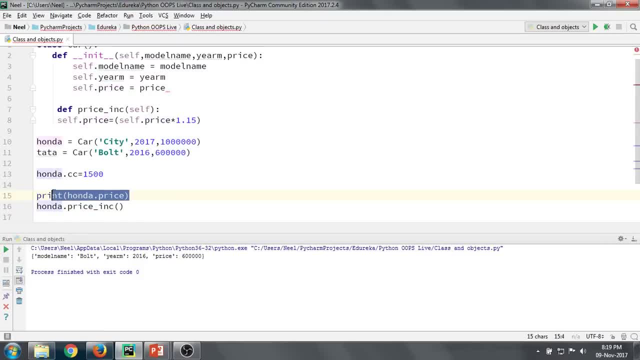 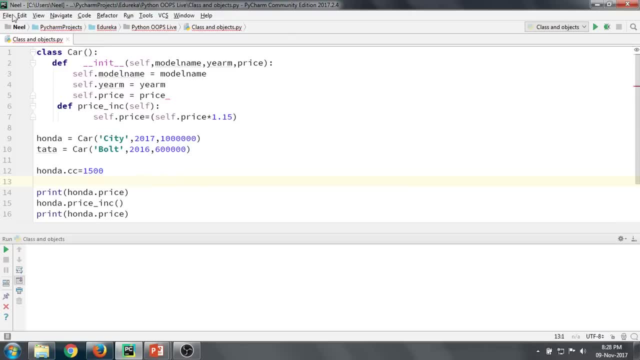 I want. ok, and again, let me copy this and paste it. ok, so, and again, see, the major issue here is it's considering this. so if you just double indent it, it's going to set back. okay, just save this and let me rerun this. ah, okay, now it's giving me the output, so it's converting it. let me just add: 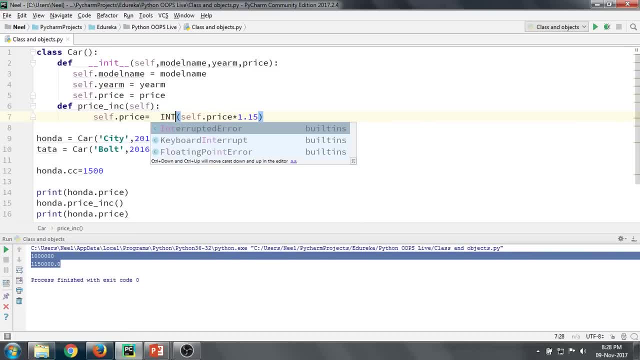 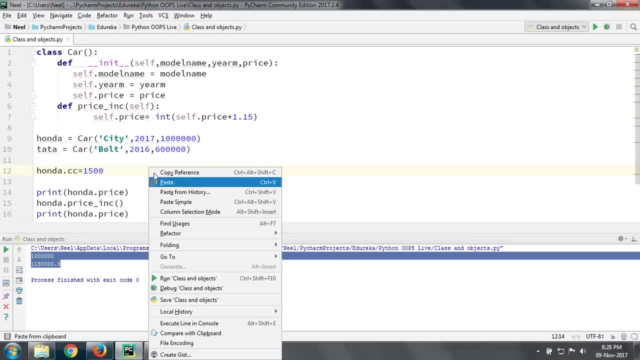 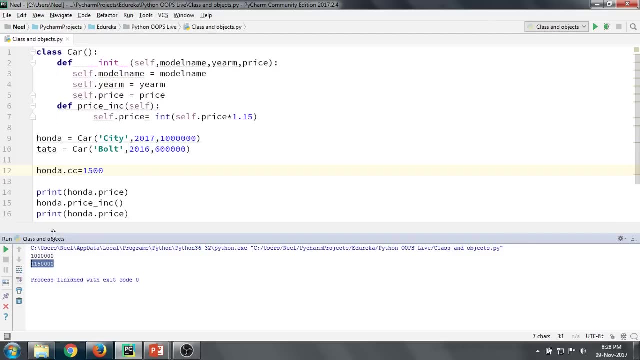 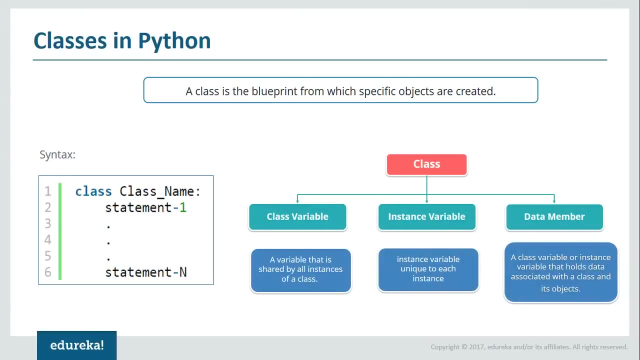 int here, just to convert it to integer type. okay, so the output should be converted to integer type for me, so it's incremented the value to 1.15 times. okay, so these are basic function operations that you can perform with respect to python. now let me go back to my presentation, and here let's. 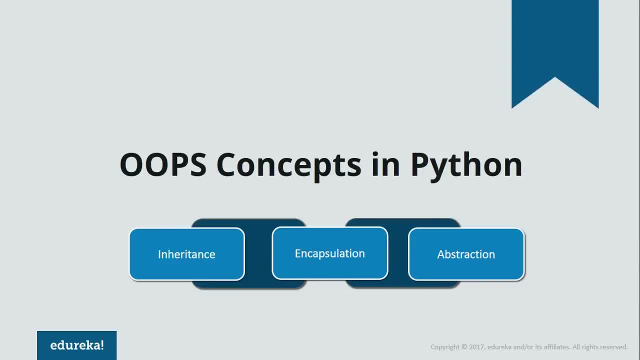 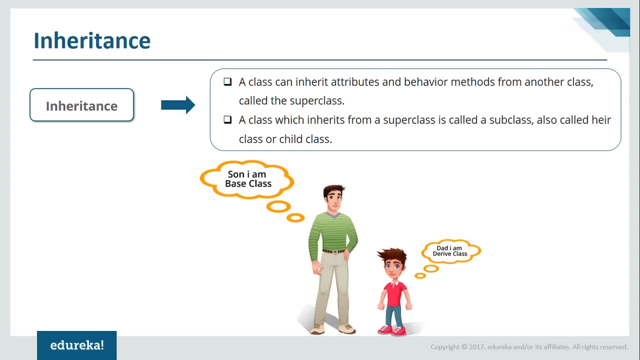 talk about the various object oriented concepts in python. now, in this session, what will be talking about are the three major concepts, which is inheritance, encapsulation and abstraction. now, when we come down to inheritance, inheritance basically is the, or the opportunity for any class to inherit the attributes and behaviors from the parent class. 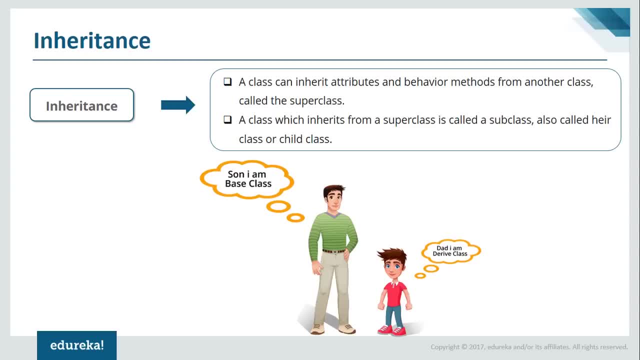 now, when i talk about a parent class, it refers to a super class as such. okay, so let's take cars itself for an example, but before that, let's look at the example here. now, your parent becomes a base class and son becomes the derived class. as such, this is same that we'll be implementing in our 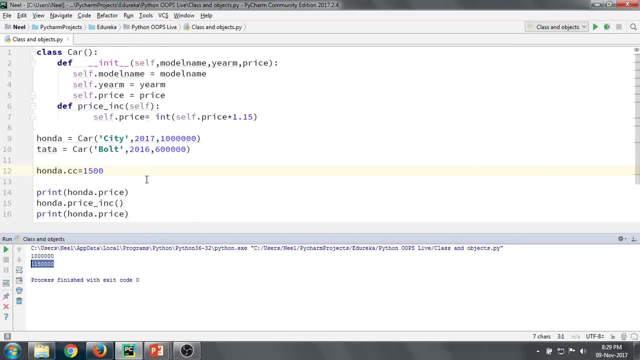 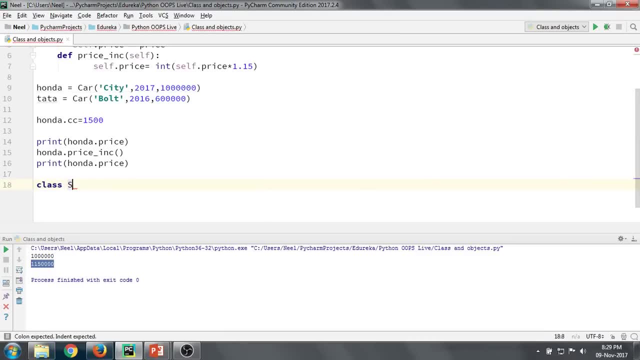 program as well. so in our pycharm what i'll do is that i'm going to create a new class and let me call it supercar. but if it has to inherit it the properties that are present in the car class, then what i need to do is that i need to specify car here. okay, that means it becomes the. 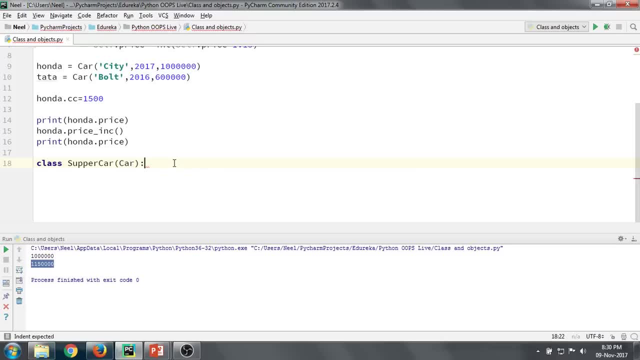 program as well. so in our pycharm, what i'll do is that i'm going to create a new class and let me parent for the supercars, okay. so here i'm not going to define anything, i'm just going to say: pass, and let me remove this from here and let me add it here. okay now, rather than making 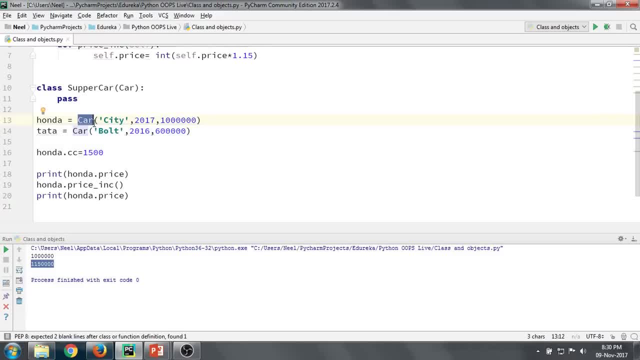 honda as a instance of car class. let me let me make it of the supercar class. okay, now, i have not defined an init operation on, nor i have i initiated the values for these variables as well. okay, so what i'm going to do is that let me just try running this. okay, let me remove this. 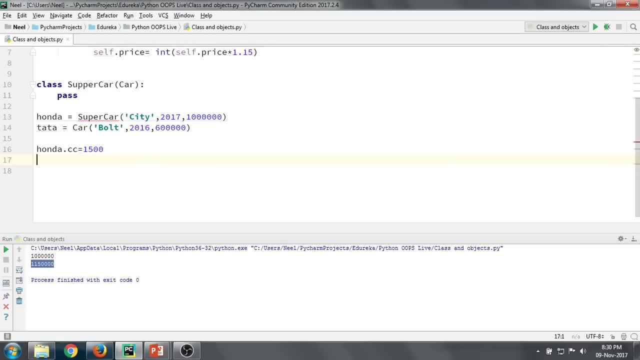 okay, and let me just print the namespace for honda, which is honda dot. okay, wait, before that let me just show you. uh, let me just print one of the values itself first, before i show you the namespace completely. let's say honda dot year. okay, so year of manufacturing is defined here. i have not explicitly defined in the child class. 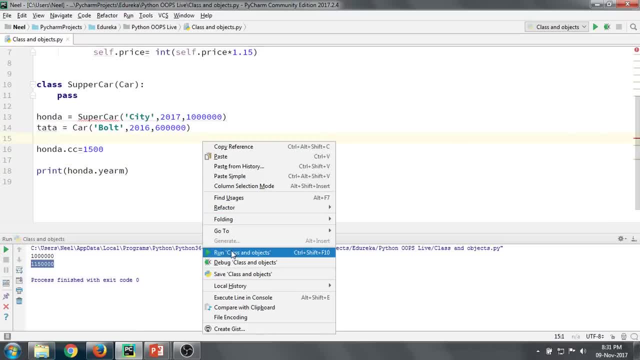 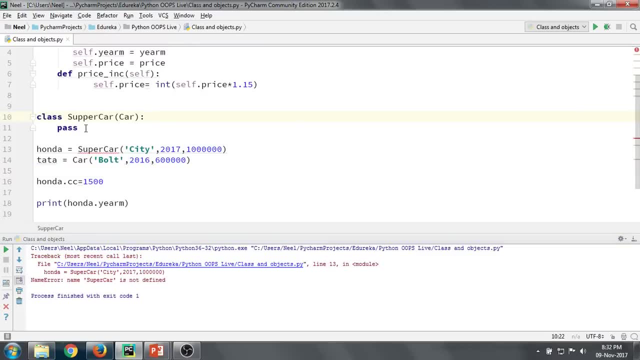 but let me make sure, let me just run this and let's see the output. okay, so here, basically, it's just passing it. ah, spelling mistake. let's rerun this now. here, what is happening is that it is referencing to its parent. okay, now to get a better understanding of what exactly is happening here. 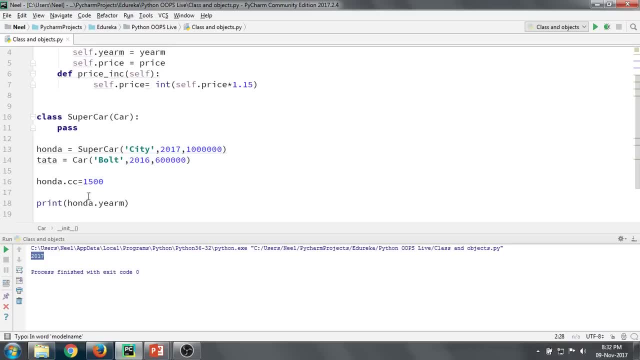 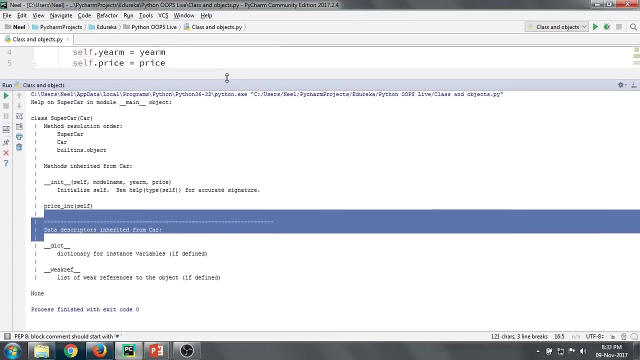 okay, we're going to use something interesting. what we're basically going to do is that we're going to argue two things. okay, so here, what is happening? here, $0.5- and here, what i'm going to do is that i'm going to pass honda. 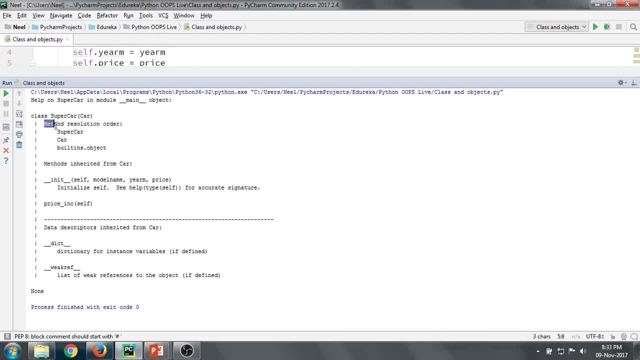 let me just comment this now. this is something that i really wanna show you guys, honda me, how it is going to follow the sequence of operations. first, it is going to check in supercar for init method, but I have not defined it here, so what it's? 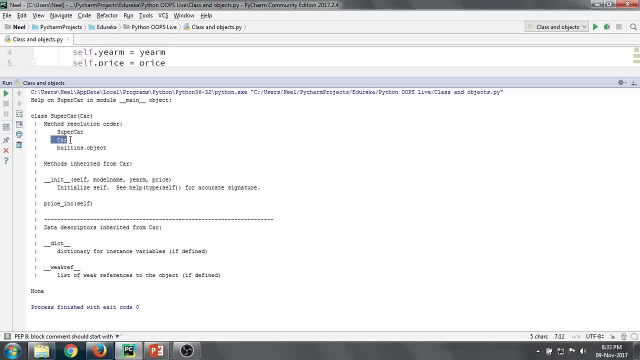 going to do is that it's going to refer the car class. if it is not defined there as well, then it will go back to the parent class for all objects which is built in dot objects. this is the parent class that is going to be inherited by. 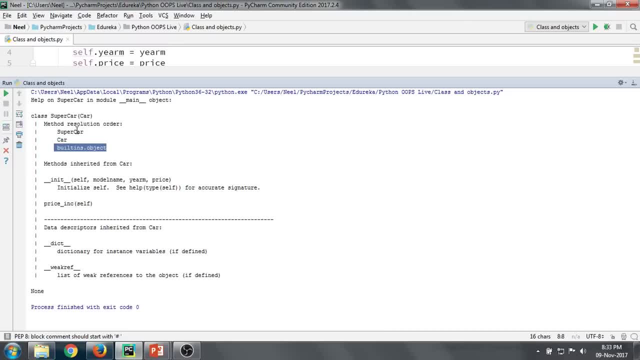 all the classes used in this language as such. so it's found the init method present in cars- okay, and it's shown methods inherited from class is the init method and it has initialized itself- okay. this is basically the sequence of operations that happen as well now when I create 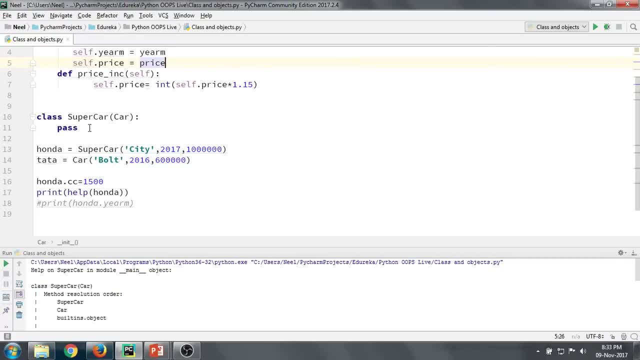 define any function with respect to the child class. it's going to check the child class. if it is not present, then it's going to check the child class which is not present and it's going to verify those, the parent class as such. Now, it can be anything as such. It can also be the price increase. 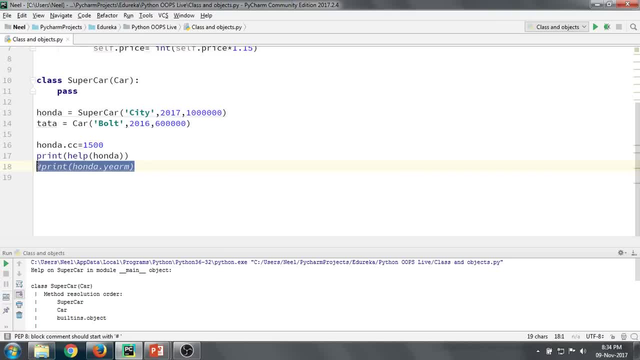 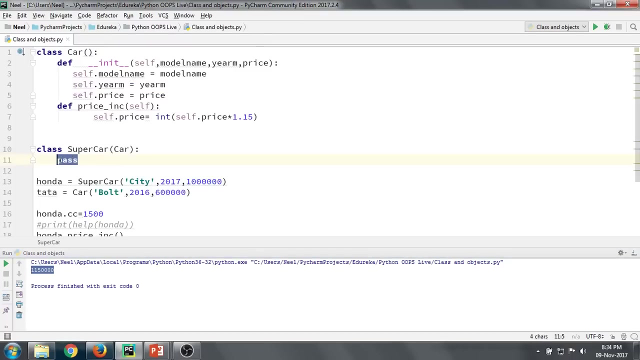 as well. Let me just comment this section out. So here again, it has inherited this method as well. Now let's say, if you do want to define an init method as part of the class, then what you basically do is that you follow. 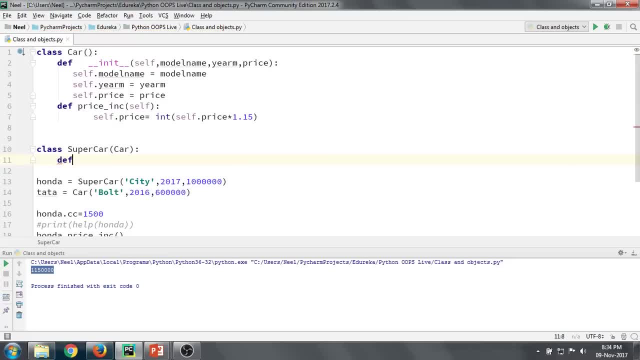 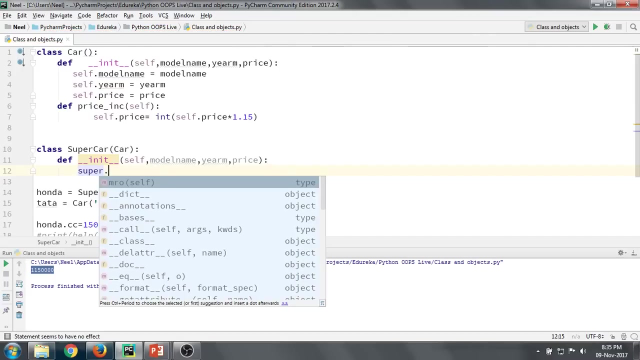 the same sequence. You write define- okay, following which you use init. Then you specify the parameters it has to take: Okay. and then what you basically do is that you shouldn't actually copy this entire code and replace it here. What you can do is that you can use the keyword superinit- Okay. 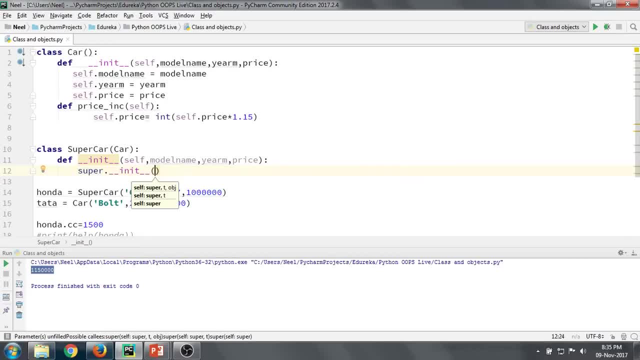 so what I'm referring to is that it should call the init function present in the super class. Okay, in that case, what I'm going to do is that I need to pass the parameters here as well. So I'm going to pass the model name, I'm going to pass the year of manufacturing. 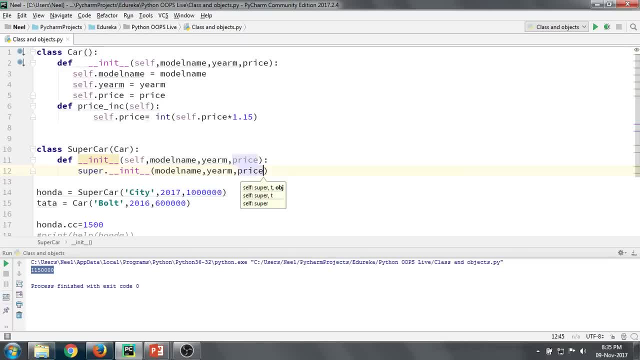 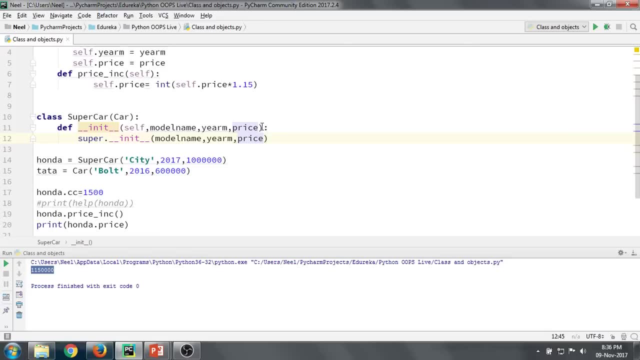 as well, as I'm going to pass the price as well. Now, this is basically to reduce the code that you're going to be writing as such. Now, apart from this, let's say, there are a few other variables that you're going to. 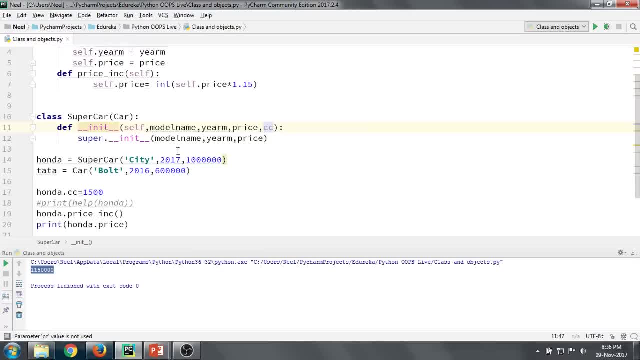 be taking. Let's say I'm going to include CC as part of my super class, Then what I can do is that I can write here: selfcc is equal to CC, So I'm basically building on what is already present and this. 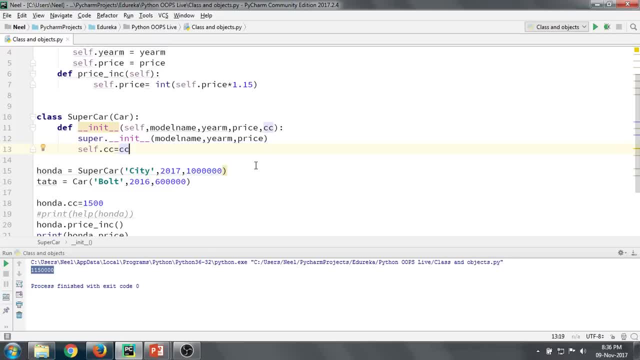 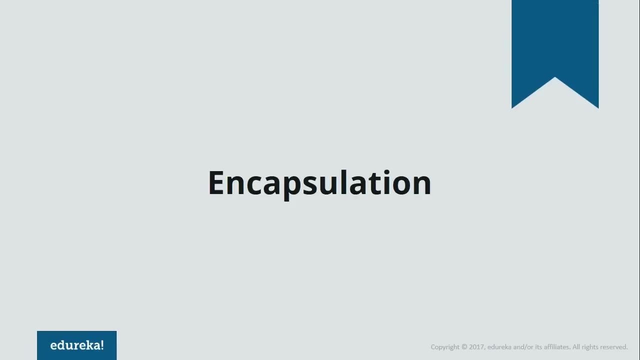 is one of the major aspects that you can use inheritance for. This in turn reduces a lot of code dependency as well, and is one of the most popular and major factor for any programming language that uses object-oriented programming systems. Okay, now coming back to the next. 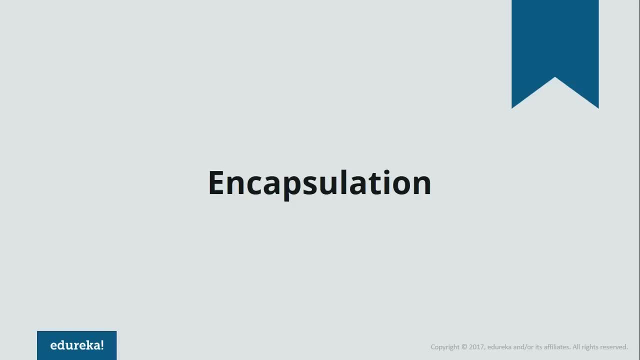 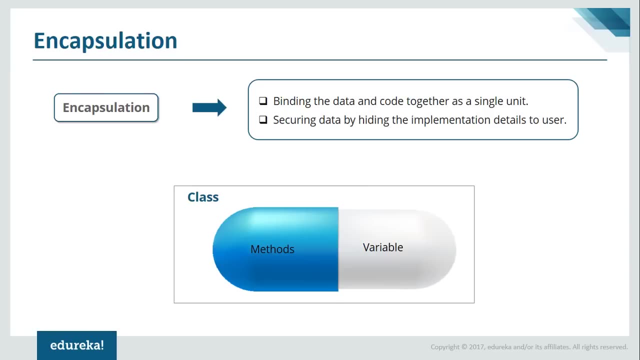 concept that is associated to Python. Okay, you have encapsulation Now. encapsulation, basically, is the method through which you bind your data and your code together. Now it also helps you in hiding your data from people whom you don't want to do it, don't want to give visibility to. So this is one. 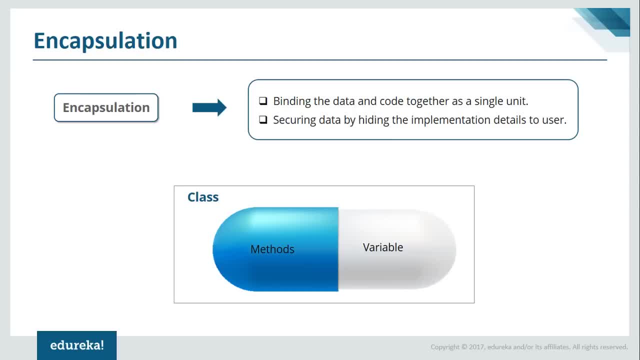 of the major key factors for any programming language as such. Now there are two major ways through which you can access or achieve encapsulation. One is by using the getter and setter method, And the next is by using at project. Okay, now we'll be talking more about that in our 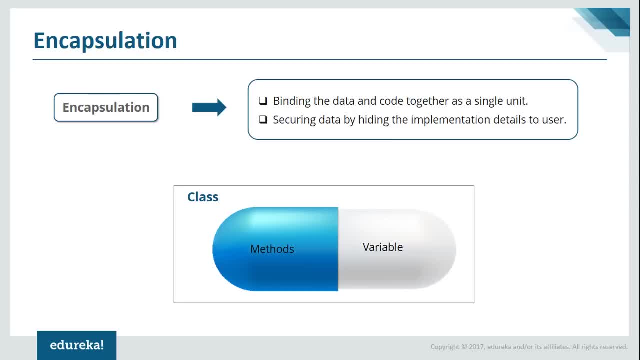 next session. But let me give you a simple understanding. What happens is that you want to change a specific value as on when in the code itself- Let's say my year of development or my year model year- just keeps changing continuously. In that case, what I need to 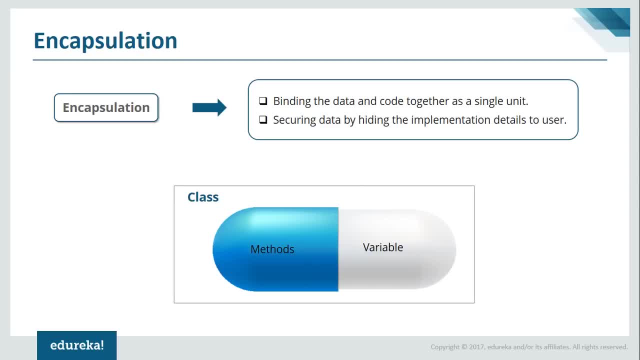 do is that I need to update these values on regular interval, But let's say there's a specific frequency on these variables ahead as well. then it becomes an issue. Same can be said with respect to price. Now price is going to be increased continuously through getter. 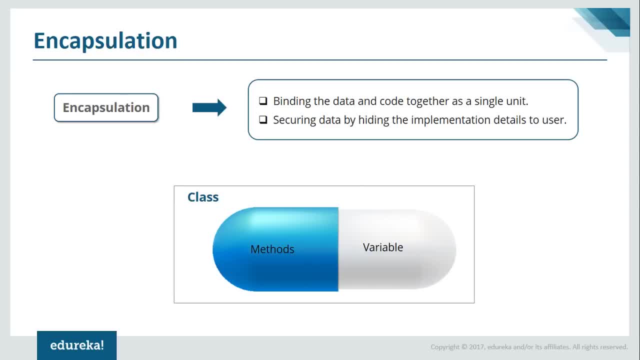 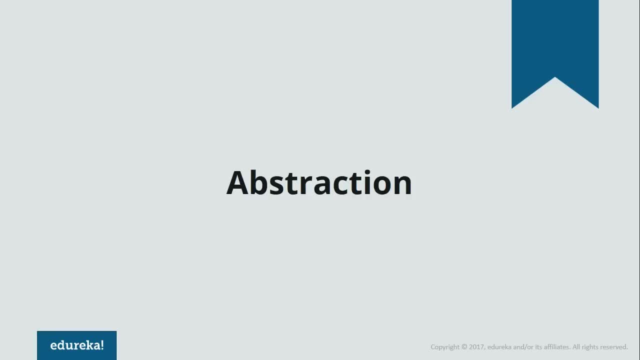 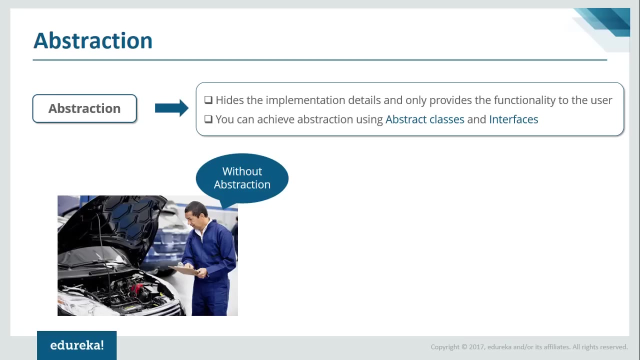 setter method. I can ensure that this is going to be implemented every time there's going to be a change as well. Apart from that, one of the major concepts with respect to object oriented programming is abstraction. Now, with respect to abstraction, what basically it means is that it hides the implementation. 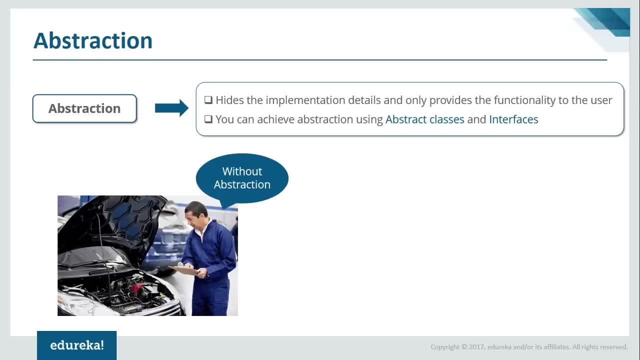 details and only provides the functionalities to the user. Now, if you look at the image here, now a mechanical engineer or an automobile engineer who works with your car is aware of the inside and out of your car as well. Now, if I need to drive a car, I don't need. 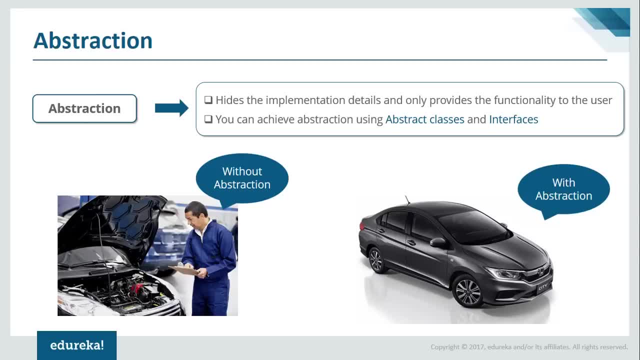 to know that. I just need to know how to turn on my car, how to change the gears and how to move forward as well. So that is what abstraction helps me achieve. I don't need to understand what exactly Happens when a gear shifts from second to third, but I just need to know that a gear 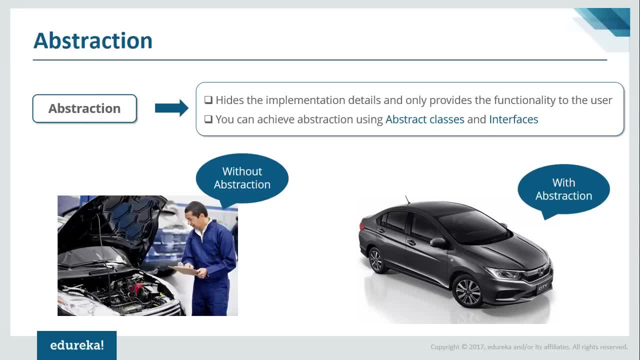 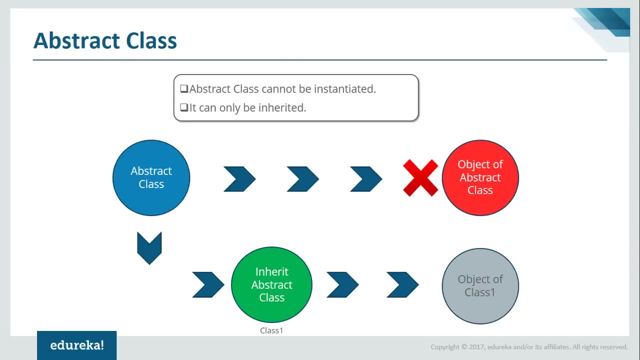 shift from second to third is going to make it easier for me to move ahead as well. Okay, so this can be achieved by using abstract classes, and an abstract class is quite similar to an actual class itself, But how is it different from an actual class? is that an abstract class? 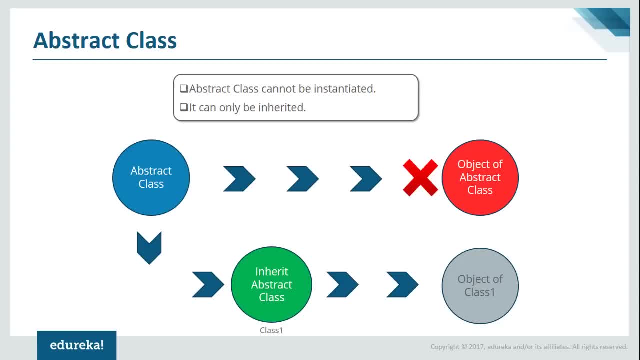 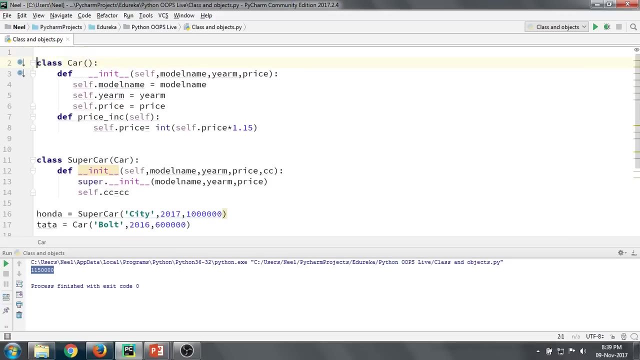 cannot have an object of itself. You need to inherit the abstract class and you need to create an object of that Abstract class as well. Now let me go back to the same example. Let's change it here. Okay, now what I'll do is that I'm going to add a few additional lines of code. Okay. 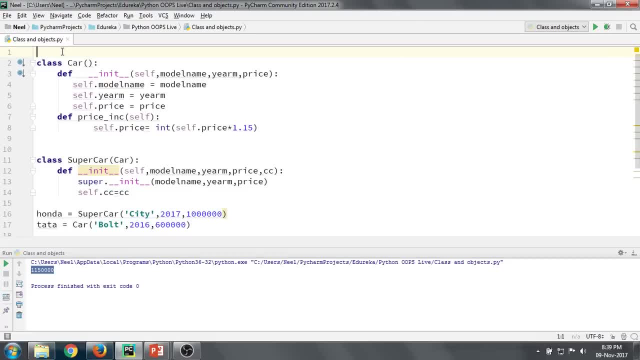 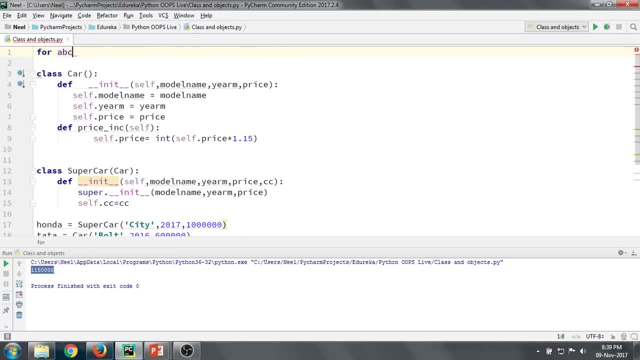 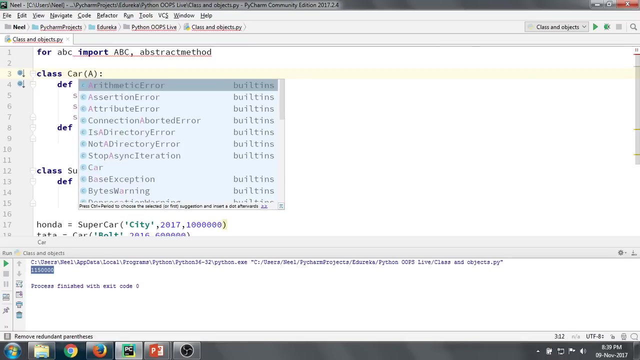 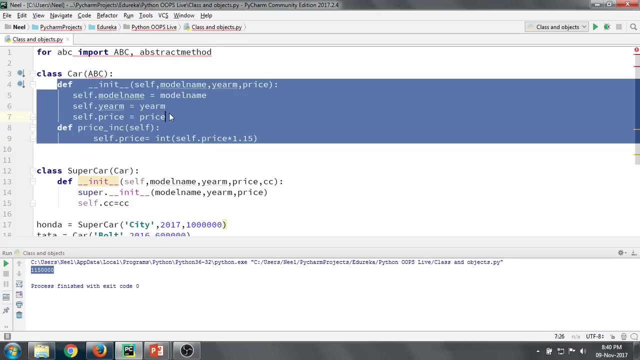 let me just copy Here. let's say I'm going to say from ABC, ABC and create abstract method. Okay, now what I'm going to say is that my car class ABC, is also inheriting this abstract. Now I'm going to remove all this and get here: 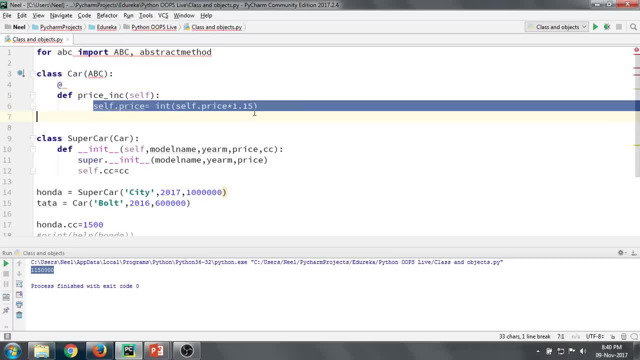 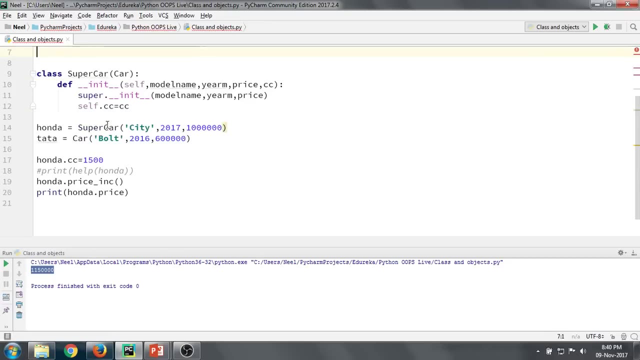 I'm going to make this an abstract method, but I'm not going to define the logic here. Okay, for now, what I'll just do is that I'll call it Okay And in my superclass, what I'll do is that I'm going to create the same function. 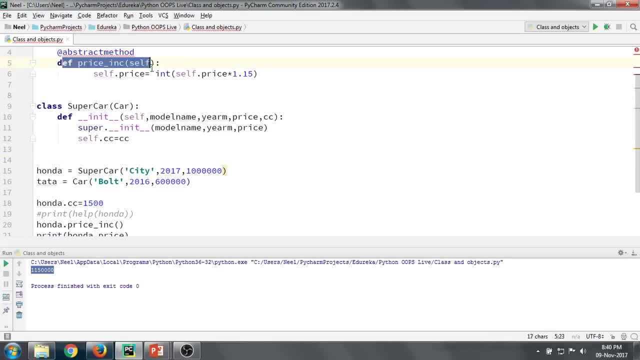 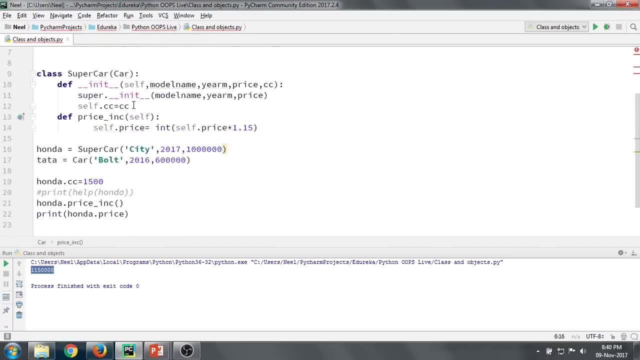 But here I'm not going to define any logic. Okay, so what I'm basically doing is that in my abstract class, I'm defining the method to increase the price, but based on my requirement. now, let's say, I don't want my superclass to have an increase of just one point, So let's.